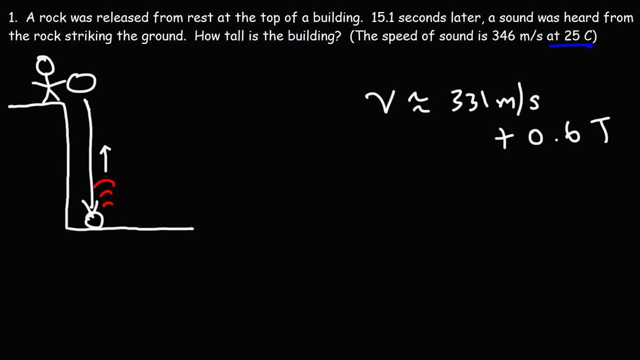 and the speed at which sound travels through air is dependent on temperature. So if you were to plug in 25 degrees Celsius into that formula, so if you type in 331 plus 0.6 times 25 in your calculator, you're going to get 346 meters per second. So that's going to be the speed of sound in this. 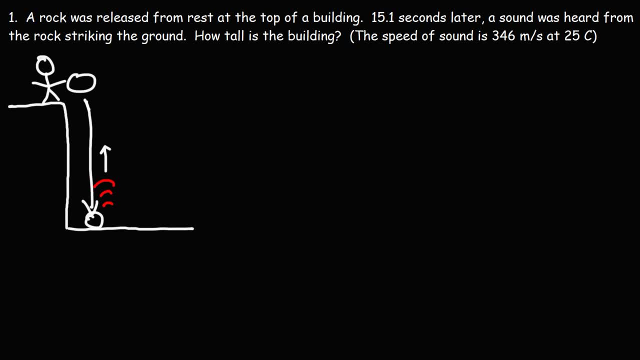 problem at that temperature. Our goal is to find the height of the building, which we'll call h. What formulas do we need in order to solve this? Now, we need to break up this problem into two parts. In the first part, the ball is falling And the time that it takes to fall. let's call it T1.. 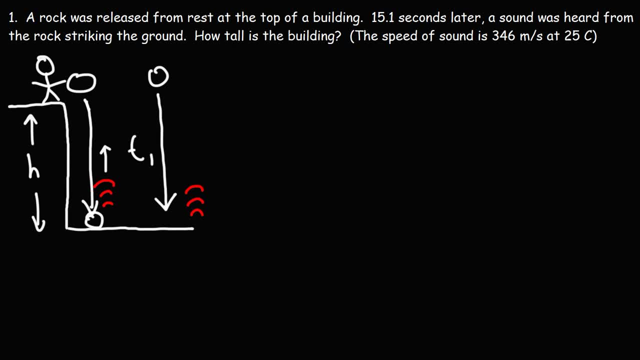 During the second part of the problem, the sound wave is traveling from the point of impact to the person's ears, And the time that it takes to fall is called T1. And the time that it takes to fall is called T1.. The time it takes for the sound wave to travel back, we'll call it T2.. The total time for this: 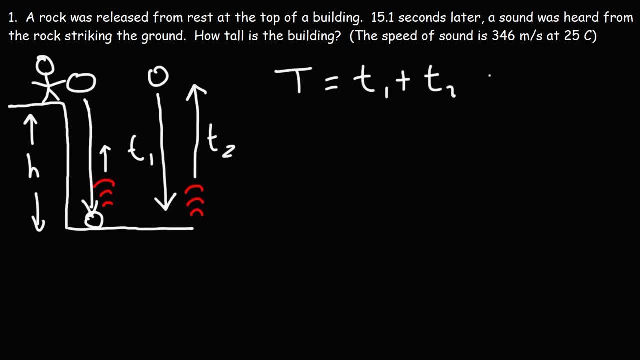 whole problem is T1 plus T2. And that's going to be equal to 15.1 seconds. So we'll save this formula for later. Whenever you get a problem like this, where you have multiple variables, you're going to need a system of equations in order to solve it, And for this particular problem, we're going to need 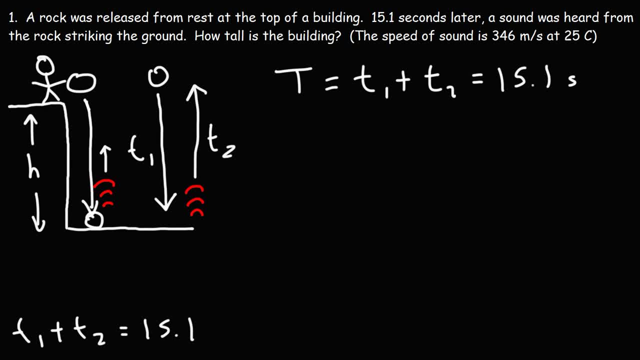 to use the quadratic equation as well, But let's save this formula. We're going to come back to it later. Now let's focus on the first part of the problem. when the ball is falling down, How can we calculate the height of the building, or at least write a formula for the height of the building? 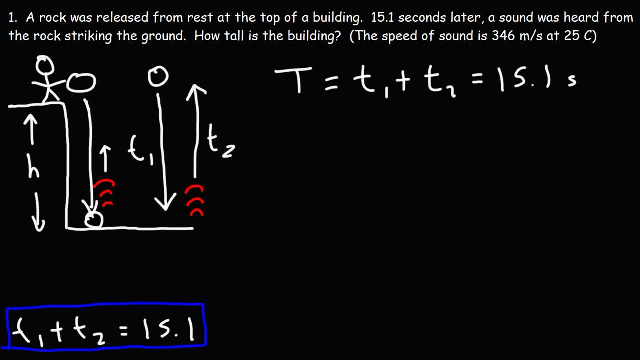 during the first part of the problem. Now, the ball is falling under the influence of gravity, So we have constant acceleration. One kinematic equation that we could use is this one. By the way, for those of you who need to know the kinematic formulas, I'm going to 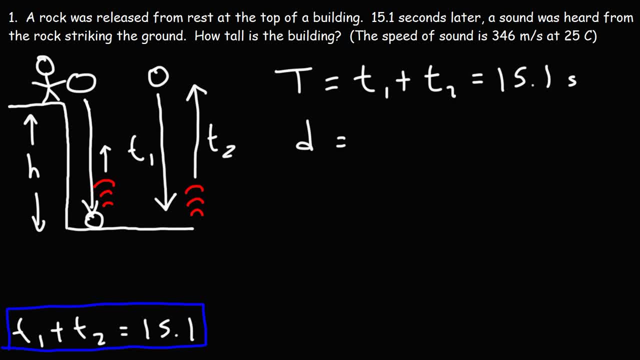 post a link in the description section below that has a video with these formulas for those of you who might be interested in it. But we're going to use this formula. The displacement is going to be equal to the initial t plus 1 half at squared. Now you could use this as displacement, You could use it as distance And you could. 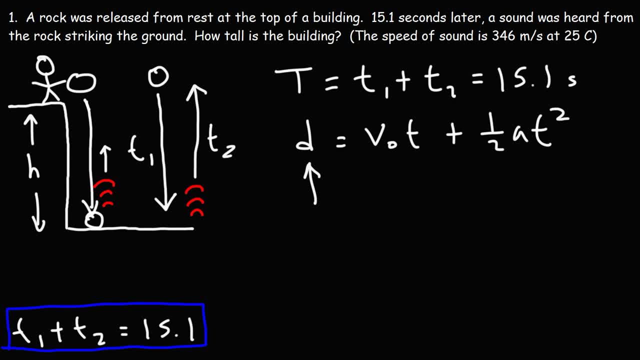 still get the right answer. If you use it as displacement, because we're going down, displacement is negative And you'll have to use a negative acceleration. If you're going to use it in terms of distance, distance is always positive, So 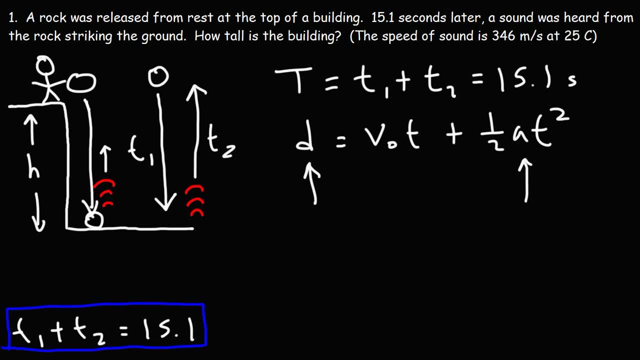 you'll have to use a positive acceleration to make that work, So just keep that in mind. So the displacement during the first part is going to be equal to the height of the building, because that's how far the ball is going to travel. 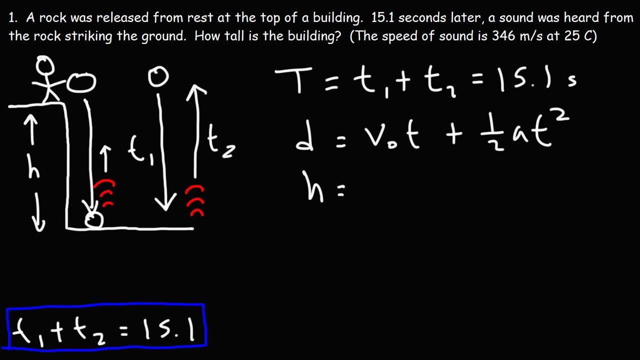 Now the initial in the y direction, because the ball is being released from rest, the initial is going to be zero. So we have: h is equal to one half at The acceleration is going to be 9.8.. That's the acceleration due to gravity. And since we're going to use a positive, 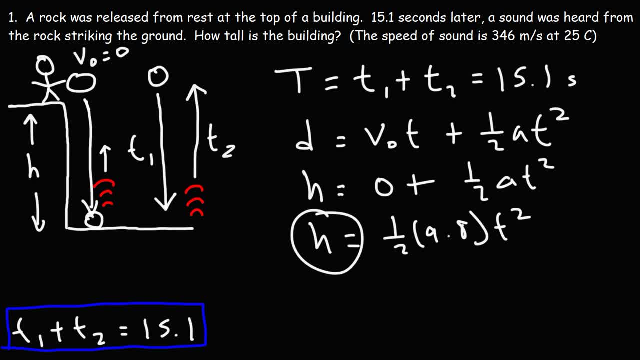 value for h, we're going to use a positive value for a as well to make this work. So we have this formula: The height of the building is going to be half of 9.8, which is 4.9 times t squared, And this is 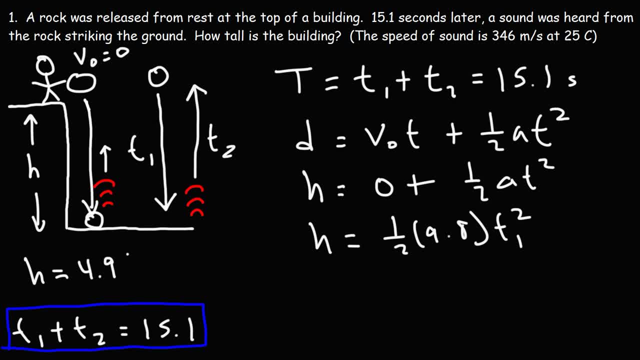 going to be t1 squared, since we're focused on the first part of the problem. So we're going to say this equation. Now let's write an equation for the second part of the problem, That is, when the sound wave is traveling back to the person's ear. 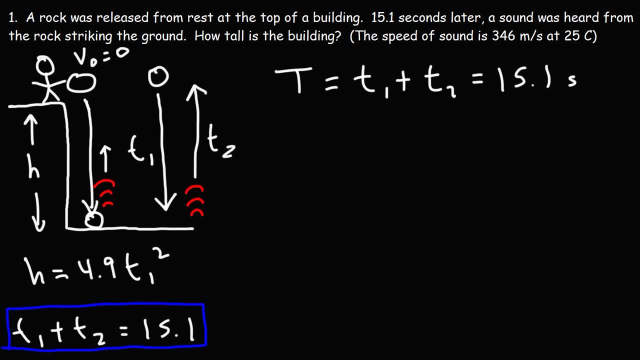 Now, the speed of sound, for the most part, is moving at constant speed. It's not accelerating. So whenever you have an object moving at constant speed, you could use this equation: The displacement is equal to the velocity, The velocity is equal to the velocity multiplied by the time, or the distance is equal to the speed multiplied by the time. 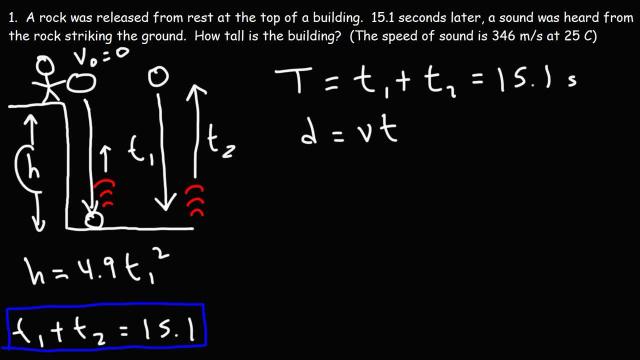 The distance traveled by the sound wave during the second part is going to be equal to the height of the building, So we can replace with h. The speed of sound is going to be 346 meters per second, And the time it takes to travel back, that's going to be t2.. 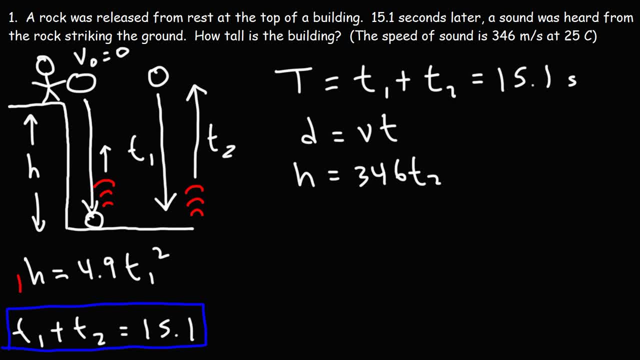 So we have this equation. So because both of these equations is equal to the height of the building, we can set them equal to each other. So 4.9 t1 squared is going to equal 346 times t2.. Now, right now we have one equation and two variables, So we got to do something about that, And that's when this equation is going to become helpful. 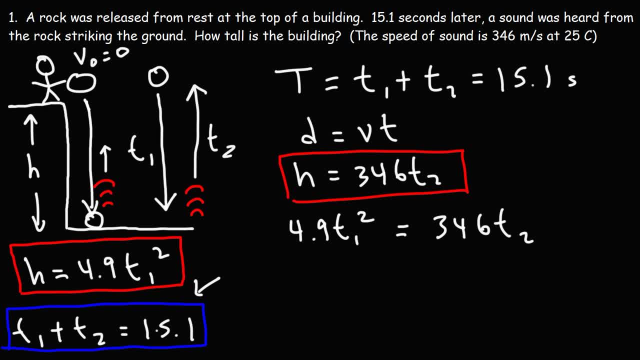 Let's solve for t2 in this equation. If we subtract both sides by t1, we'll get that t2 is equal to 15.1 minus t1.. Now what I'm going to do is I'm going to replace t2 with what it's equal to there: 15.1 minus t1.. 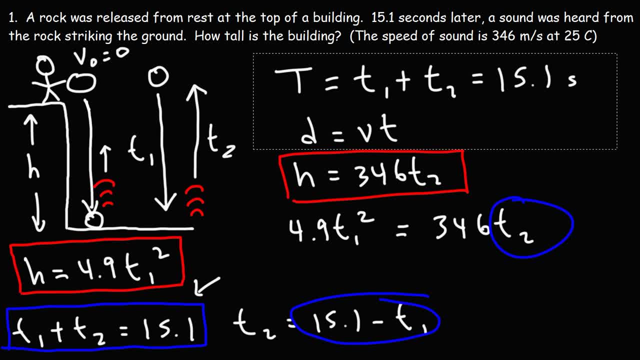 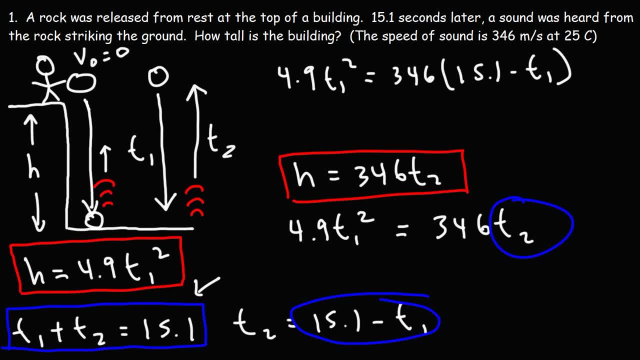 so now let's solve for T1, but first we need to distribute. so let's distribute the 346, 346 times 15.1, that's 5224.6, and then this is going to be minus 346 T1. so notice that we have a quadratic equation. 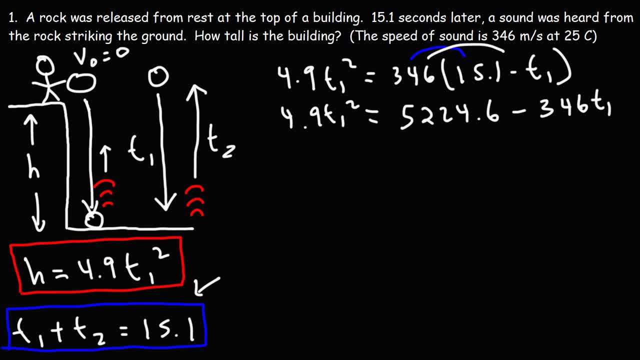 and we need to put this equation in standard form. so I'm going to take all the terms on the right side and move it to the left side, so moving this term to the other side. it's negative on the right side. it's going to be positive on the left side. 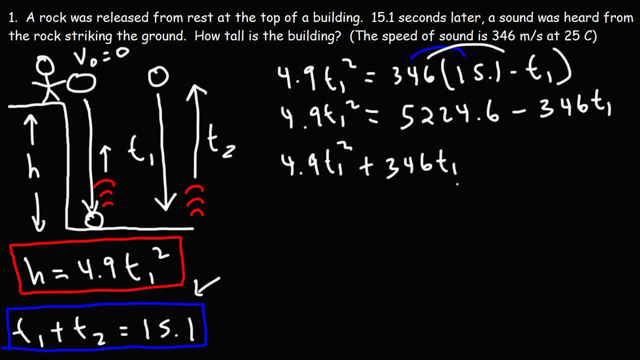 and moving this term as well. it's positive on the right, but it's going to be negative on the left side. so now we have this equation and, as you can see, it's in standard form of a quadratic equation: ax squared plus bx plus c is equal to 0. 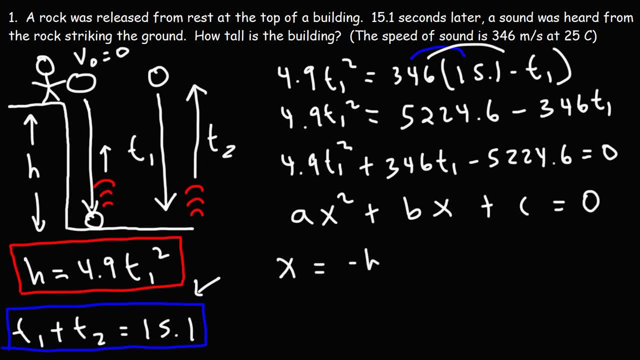 and here's the quadratic formula: x is equal to negative bx plus or minus the square root of b squared minus 4ac divided by 2a. but instead of x this is going to be T1, so T1 is in place of x in this problem. 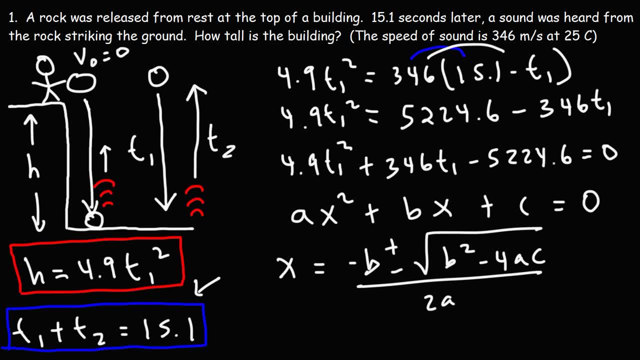 so T1 is going to be equal to negative b. b is the number of x in front of T1, so b is 346, a is 4.9 and c is that number. so this is going to be negative 346 plus or minus the square root. 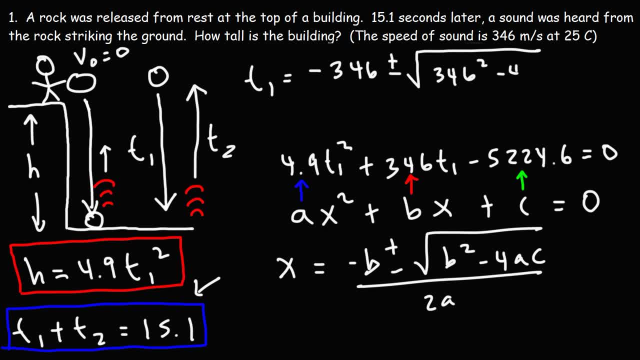 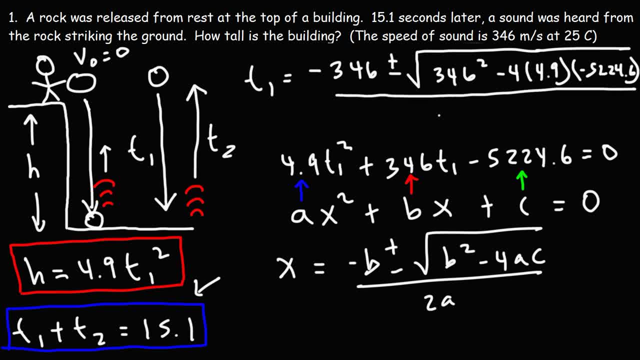 and then c is 4.9- I could use a bigger screen here- and then, divided by 2 times a, a is 4.9. so I'm going to simplify this first: 346 squared minus 4 times 4.9 times negative 52. 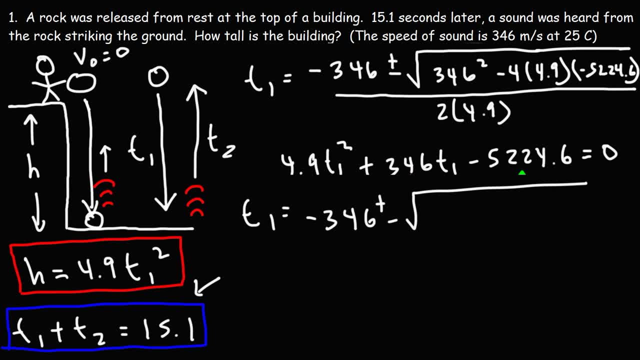 24.6. so I got this number, 222,118.16, and this is going to be divided by 9.8 and if you take the square root of that number, you should get 471.294. now we're going to get two possible answers here. 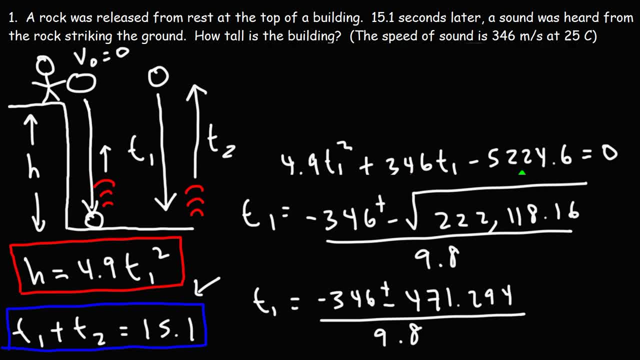 so the first one, we need to use the positive sign, and for the second one we'll use the negative sign. negative 346 plus 471.294 divided by 9.8, so you should get 12.785, 7.85 seconds. now for the other answer. 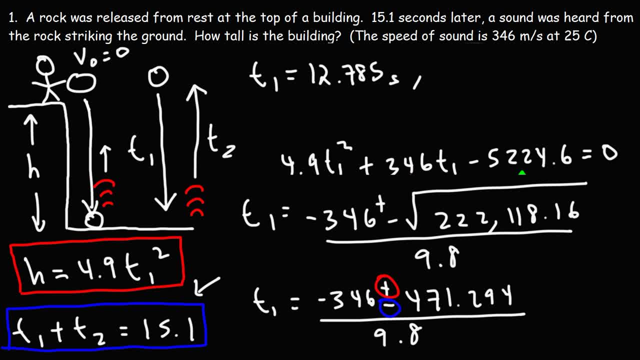 we need to use the negative sign: negative 346 minus 471.294 and then if you divide that by 9.8 you'll get negative 83.397 seconds, and of course time shouldn't be negative. so we could scratch that answer, we could eliminate it. 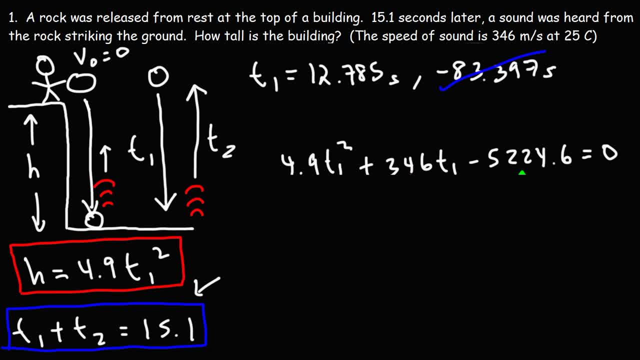 so now we have our value for t1 and if you want to check to make sure it's correct, you can plug it back into the original formula. but now let's take this answer and let's calculate the height of the building. so it's going to be: 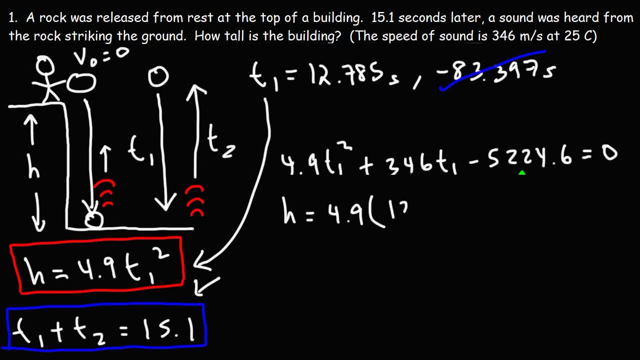 4.9 times t1 squared, or 12.785 squared the height of the building. so I got 800.9 meters. so we could say the height of the building is approximately 800 meters. now we can also calculate it using the other formula.